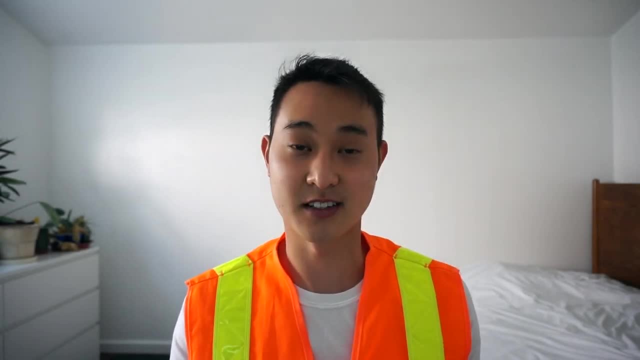 really confused as to like what we did, because I thought that that was what we only did. Like that was what I thought that only environmental engineers did, for you know all fields But in reality it's not true. In different companies, you could be doing different things even though you. 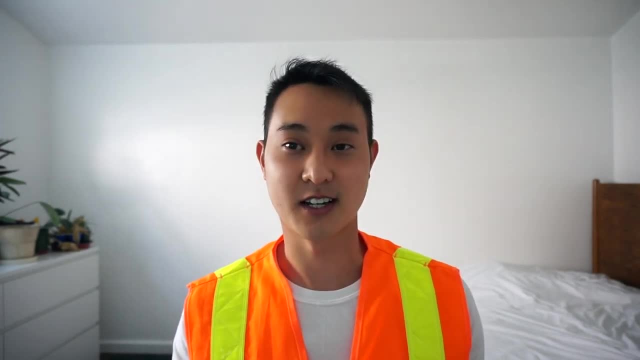 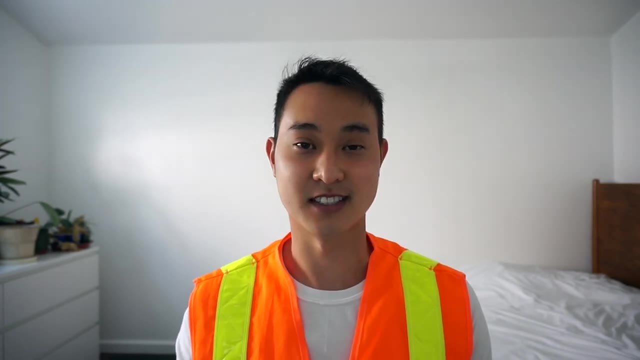 have like the same title as an environmental engineer. So I wanted to clarify and prove that you know, as an environmental engineer- that title, you have many different aspects that you can go into. So, according to LinkedIn, what I see is you know as I'm going down the job search page that 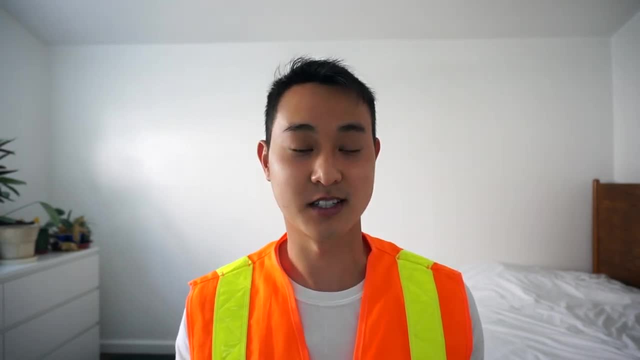 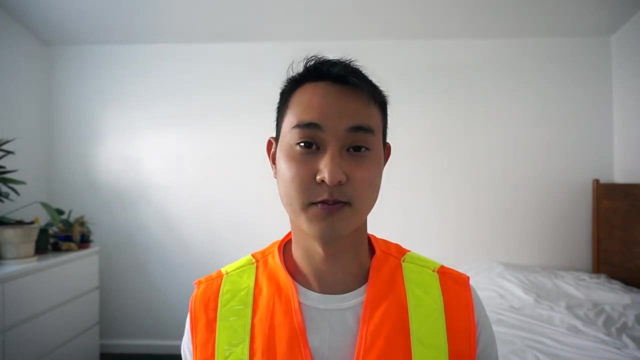 environmental engineers. they can do a lot of different things And, yes, some things are, you know, similar and relative to what I do. I just want to point out that you can be doing a lot of different things in many different fields, Many different aspects, ranging from, like, what I do. 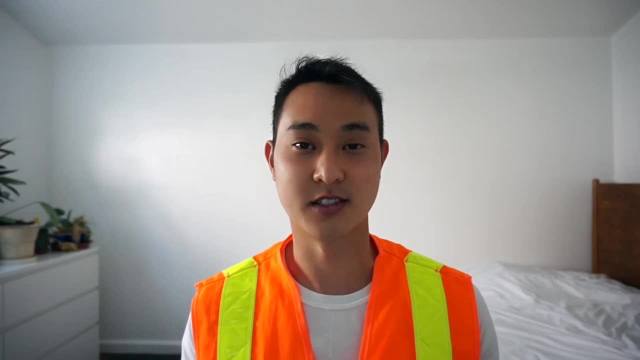 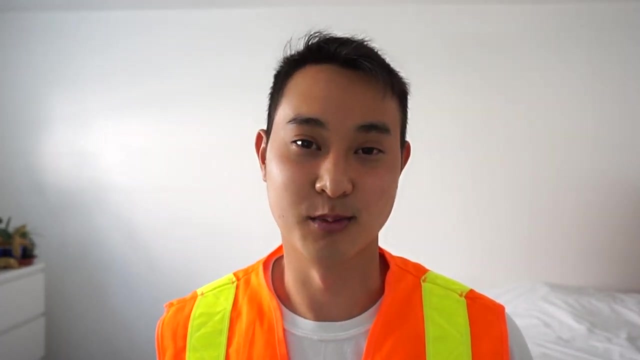 environmental compliance, or research and development, Or health and safety, Yeah, so basically I just want to go over, like as I'm scrolling through LinkedIn, always on my feed, what we do And, as you can see, I'm actually wearing like my official, I guess- inspection clothing, rather than just the normal blue shirt that I typically wear, I guess. 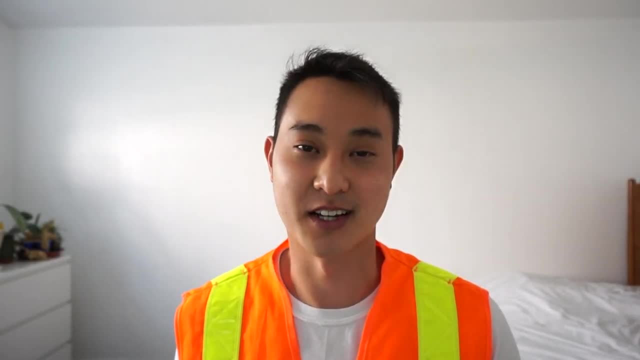 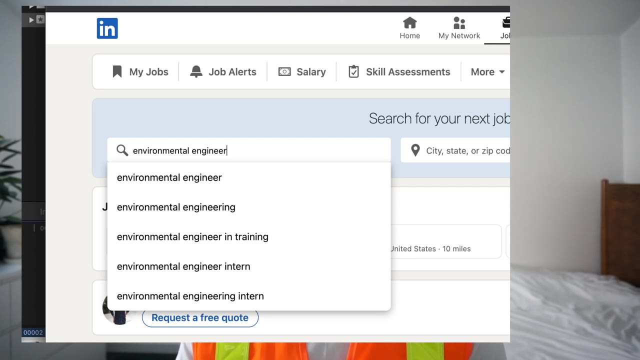 it makes me feel more authentic and maybe you believe me that I am actually an engineer if I'm wearing something that looks like engineer clothes. So, basically, I'm going to log into my LinkedIn, Click the jobs tab and just type in my name. I'm going to type in my name. I'm going to 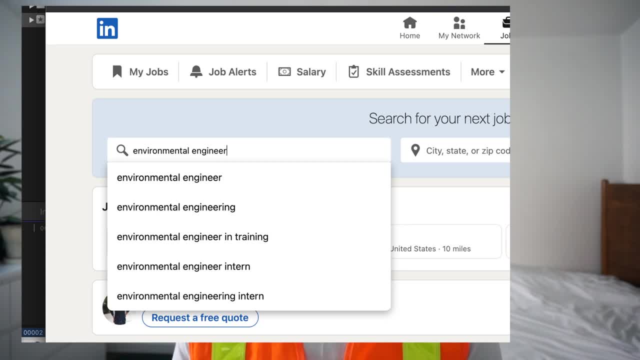 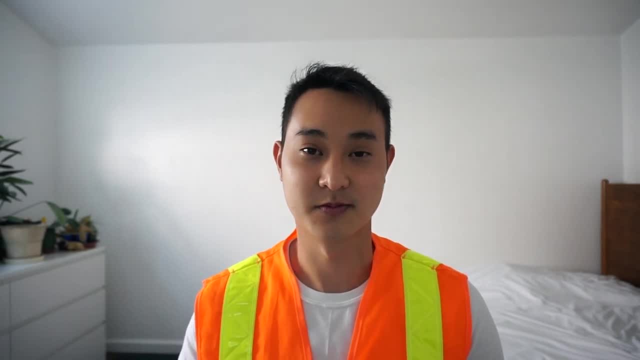 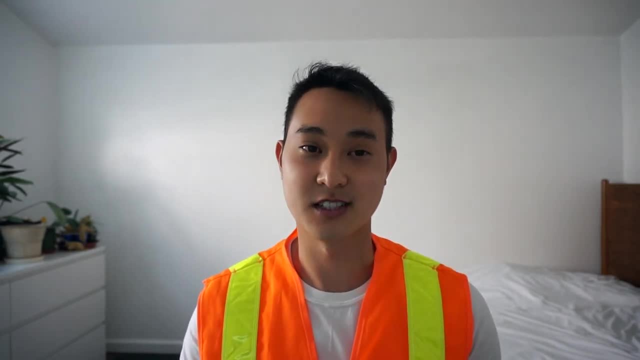 or it could be like environmental compliance or you know some sort of relative similar position that has like the same responsibilities as an environmental engineer near my location. So as you're searching for this job, you might have different pop-ups, different positions, different companies, different- you know job titles that is like relative to your experience. 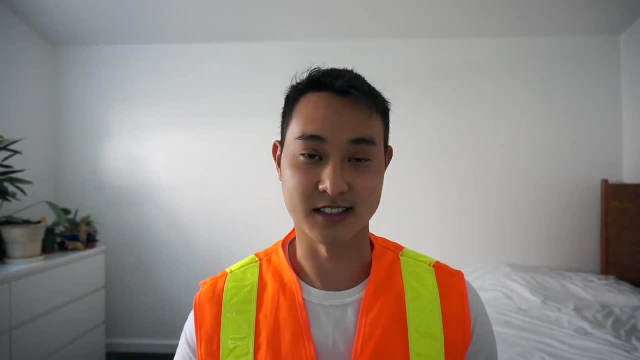 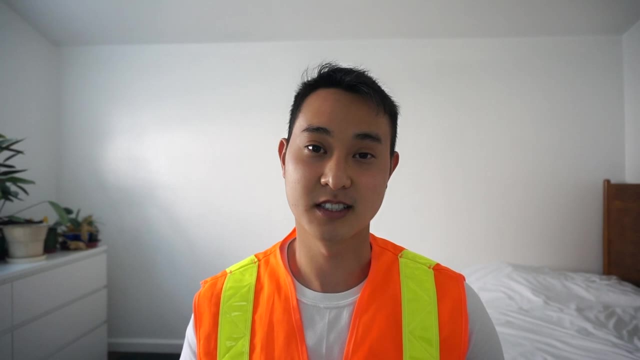 And relative to your title search. But you're going to see what I see at least, And again, these companies will probably not appear on your job search. So you're going to see the company, You're going to see the responsibilities, You're going to see, like, maybe the benefits and so on, Like really, 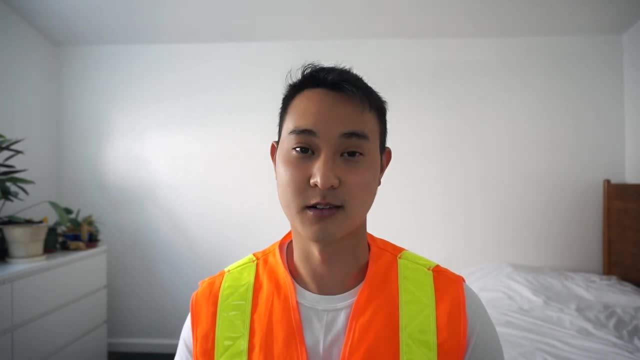 what's the responsibilities and duties that they're looking for, And I'll give my comments and feedback. what or how relative, how true that is, how relatable that is, and probably what you're expecting when you're like looking for this job. Alright, so the first one that I see is an entry. 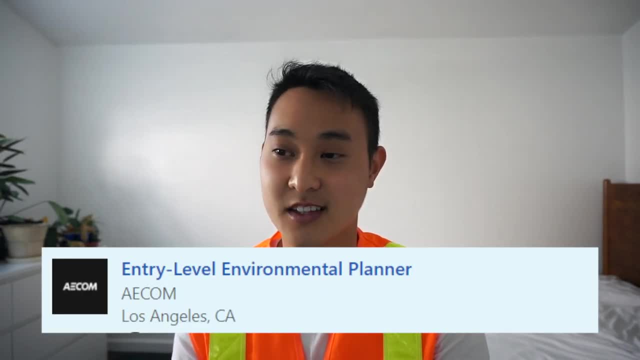 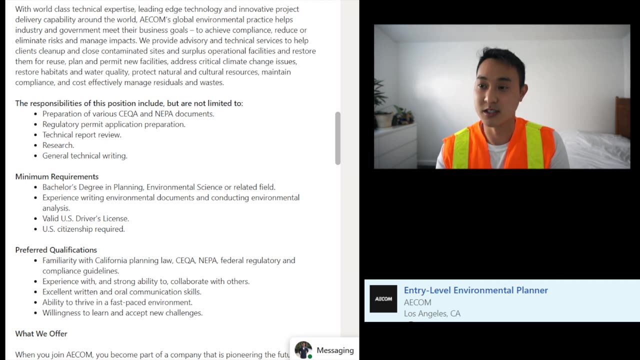 level environmental planner from AE. I'm going to type in my name. I'm going to type in my name. I'm from AECOM, near Los Angeles, California. So you know just my location. I'm just going to go and skip right ahead to the responsibilities. The first little point is preparation of various 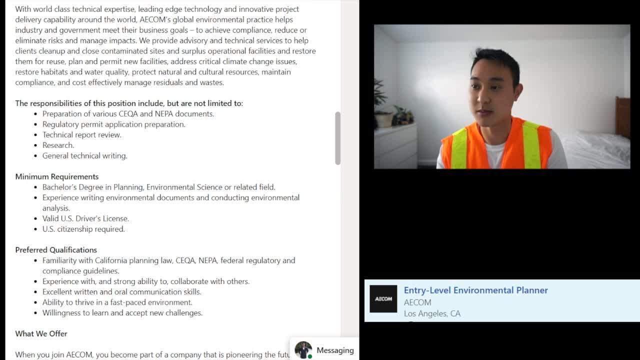 CEQA and NEPA documents: Regulatory permit application preparation, Technical report review, Research, general technical writing. Minimum requirements is, you know, bachelor's in environmental science or, like some relative field, Experience writing environmental documents. You know conducting environmental analysis. You need a driver's license, so you're probably going. 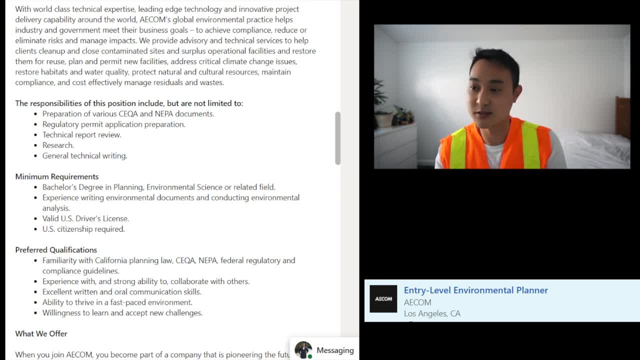 around the field a lot Preferred qualifications. You got to be familiar with California, So specifically our state, CEQA, NEPA, federal regulatory guidelines. You know experience and strong ability to collaborate with others, because you know you're going to be talking to a lot of. 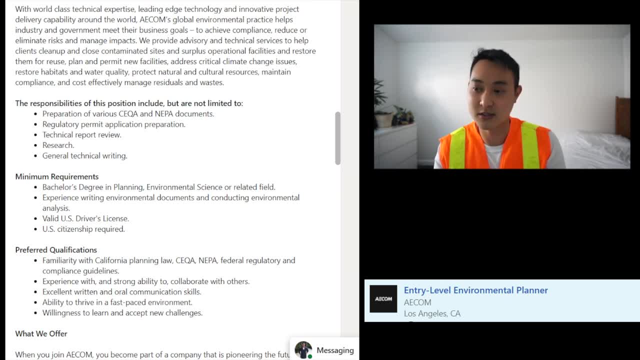 people: Excellent writing and communication skills, Ability to thrive in a fast-paced environment, You know, willingness to learn, Just like a general, like good to do, Good personal development Habits. So my thoughts, I mean this is sort of what I do at my work, Although I'm not like directly. 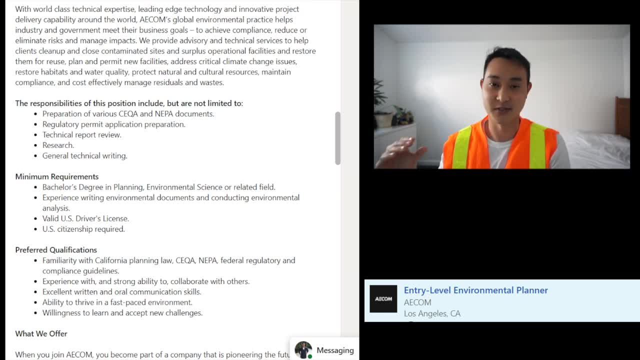 focused into like NEPA writing. Like you know, these are different fields, Different aspects and different specific categories. Again, what I do is like hazardous waste, Hazardous materials, Solid waste, recycling, And I do do some like reporting, But I don't like, it's not my. 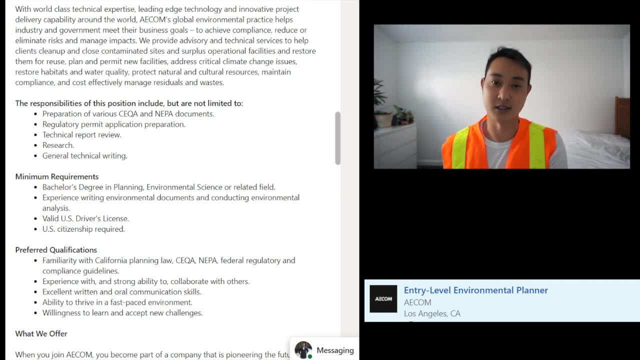 responsibility to do the NEPA reporting. It's someone else's Another- co-workers, basically. But I understand what they have to do. I just don't do it often. So right off the bat I see like permit application preparation, writing For my composition, I don't have to like write permits. 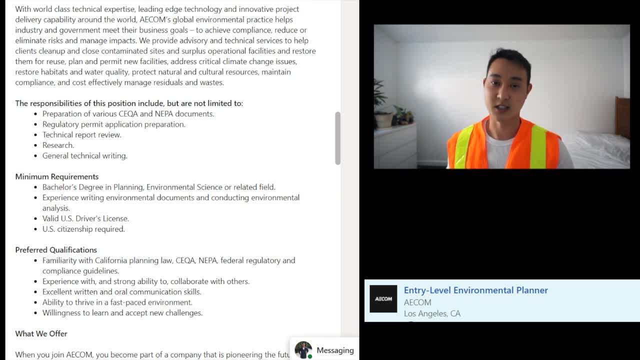 I've heard of a lot of people having to deal with permit writing. Yes, we do deal with, like federal agencies, NEPA and those things, But again, it's not my role, It's just someone else's role. So, relative to my position, this is pretty much what I expect And what you probably will be doing if 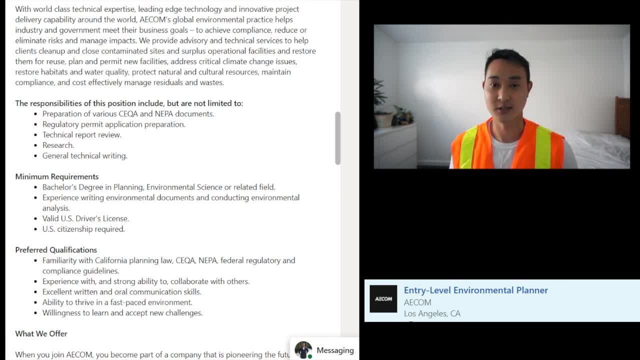 you are into, like you know that field. So so far, so good. I am, I guess, like if I were to apply to this job, I can probably get it because I have experience And I know what they're doing. I learned so much of it myself, But I at least know what they're doing. So this one is an environmental 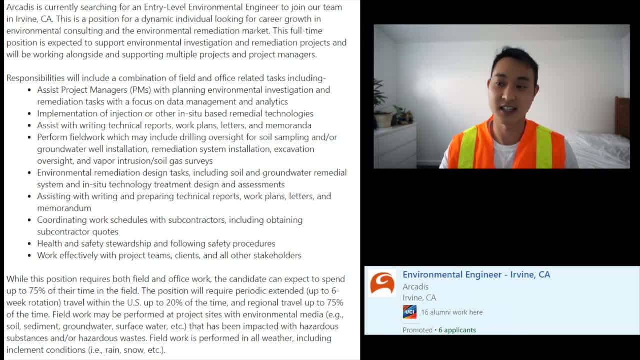 engineer in Irvine, California, from company Arcadis. Jumping straight into their responsibilities, It is to assist project managers with planning environmental investigation and remediation tasks. Implementation of injection or other in situ based remedial technologies. Assist with written technical reports- So get more writing. Perform field work, which may include drill. 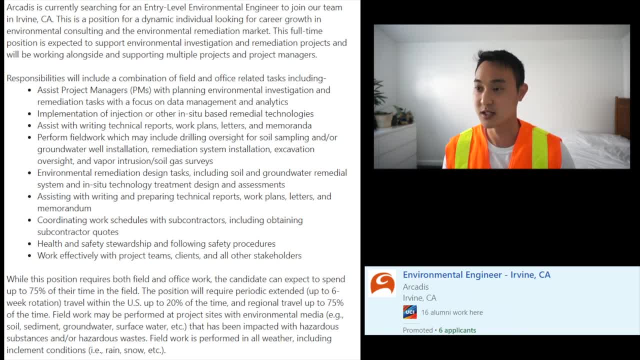 oversight for soil sampling and or groundwater well installation Remediation system installation Get into the next one: Environmental remediation design tasks. Assist with writing and preparing technical reports, Coordinating work schedules with subcontractors, Health and safety stewardship Work. 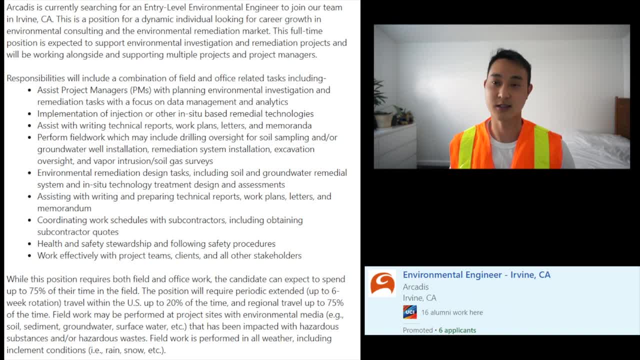 effectively with project teams. So the first part is like helping project managers, Probably construction workers, Like basically overseeing that site and saying, like you know what do you have to do and how can I help you do it- Injection or implementing remedial technologies. So this is 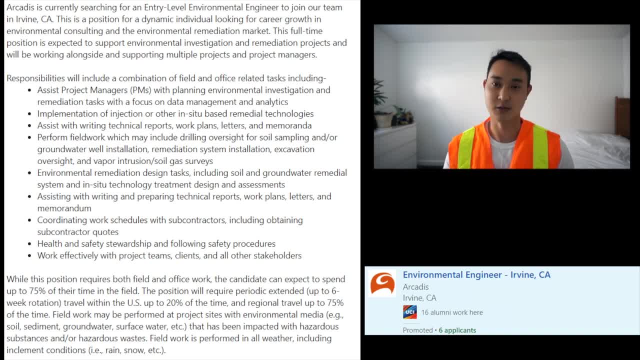 where I sort of don't do this. It's just not within my like scope of work or like my responsibilities at my current work. What I see is that they're Probably gonna be at that site, So like, let's say, you have bare ground dirt And so they want you. 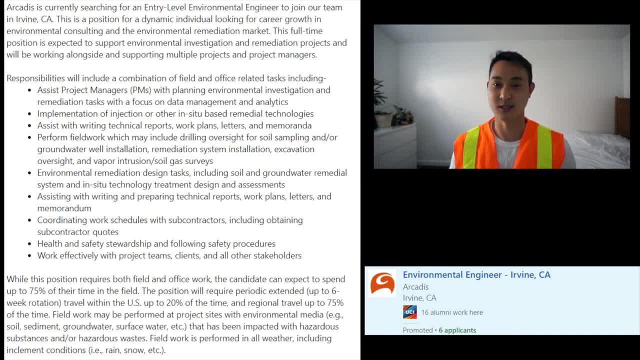 as an environmental engineer to show up there and like: get a sample of that dirt. So you might just get like a jar or like a shovel and just like dig up some dirt, Compact that, Put it in a lab and say: here's your soil sample, Here's what you're gonna be working with. You know before you even start. 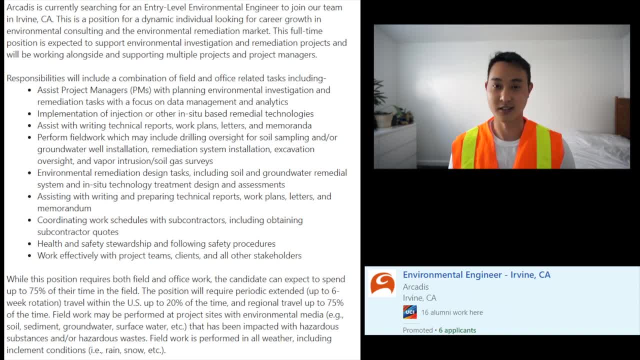 like getting a big tractor and start like digging up ground. Here's the soil, Here's what you're gonna be working with. You know it might be difficult, because it's very compact soil or something. because the soil is very, you know, brutal, It could just collapse. So that's why I 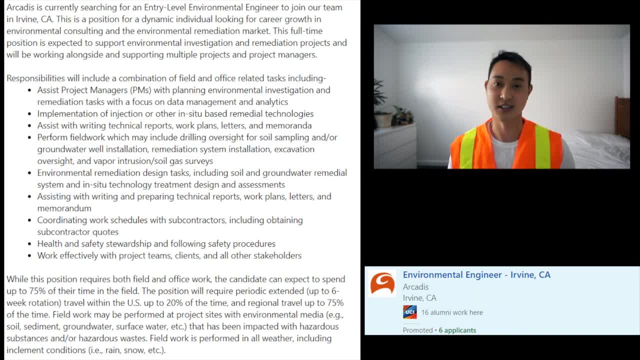 have you come out and like: test it before you know someone gets hurt. So that's where like soil sampling comes in Before the start of the project and environmental remediation. That means that something bad happened. You know, maybe something spilled. So now they have to like: 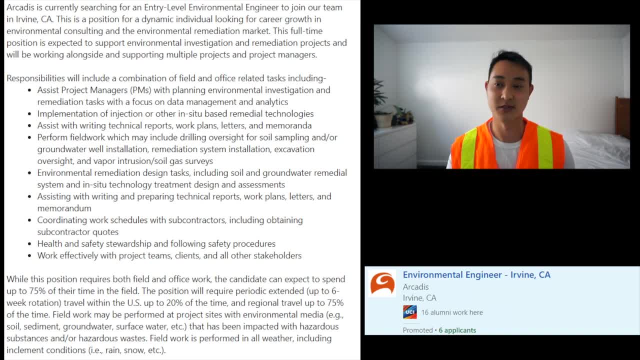 clean it up, So they might have you come out and like say, here's a problem, Can you fix it for us? Like, what do we have to do to make the soil not toxic, You know, not poisonous? So again, this is far off from what I do. I don't do soil sampling. I don't do remediation as part of my work, Although 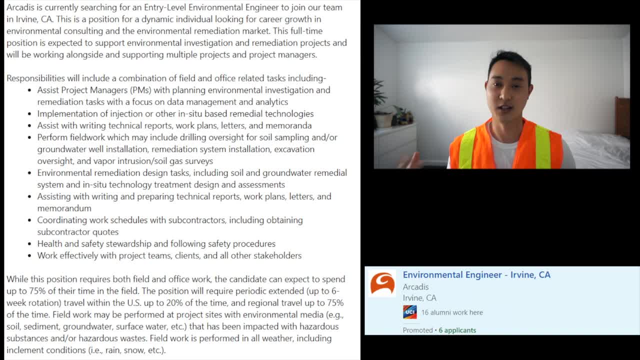 I know people- or at least for my work- we have other people do that, Like we have subcontractors or other. you know we hire other people to do that for us Because, like, we're not, I guess, professional on that, But as part of what I do, Yes, I do go out in the field sometimes I do talk. 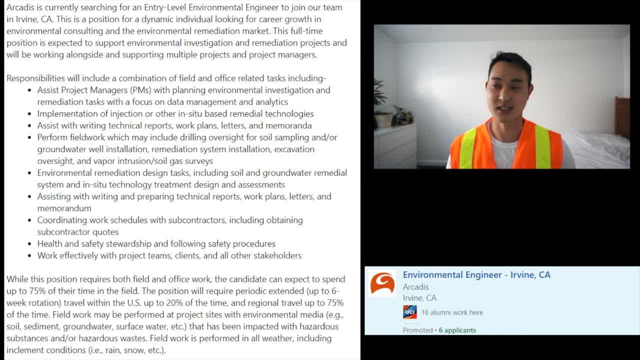 to those construction project managers and say, hey, make sure that you're safe. Did you guys have a plan, you know? before you started digging up dirt, More than likely coordinated with them and said that, okay, before you start digging it up, you know, here's what you. 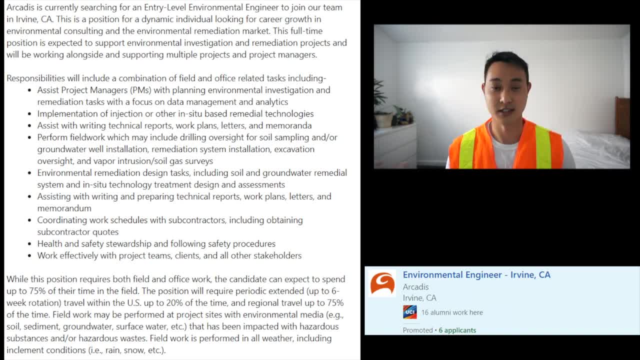 can be working with. Here's some possible problems that might happen. Or here is a problem, So you know, here's the money. Find someone who can fix a problem for you before you start working on it And then creating some other, bigger problem, And the other responsibilities are the same- old you. 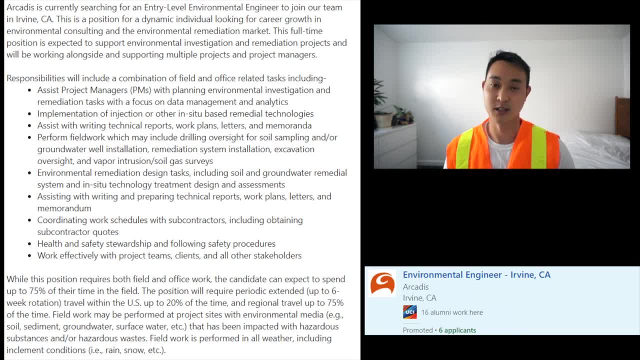 know, just writing reports, Tactical reports and like working with other people, Just, you know, making sure that people can actually follow the rules. And underneath that, responsibilities it says that you can be traveling a lot. I think 75 percent of the time I'm just in the field, So I can see this entry level position is more towards like field work. 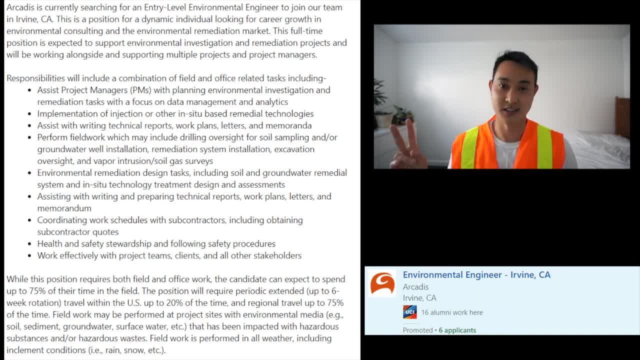 So you're not going to be in the office most of the time. You're going to be out in the field or out, you know, in that construction site Just looking at dirt, saying, okay, here's what you got to do, And you're just talking to people. So less on paperwork, More so on actual talking to people. 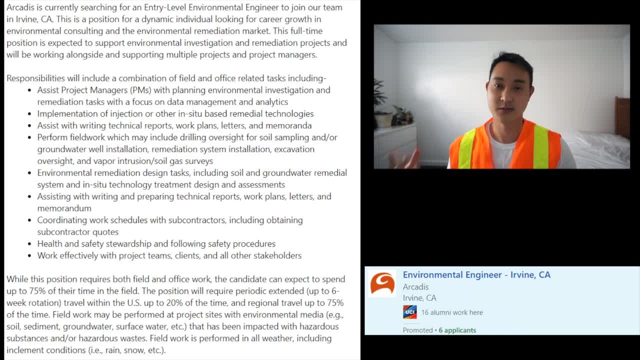 and like getting your hands dirty. If I were to apply to this job currently, with my current knowledge, I'm, you know, 50- 50. I might not get it Because I don't have that much field work. They're saying like 75 percent of the time you're going to be in the field. 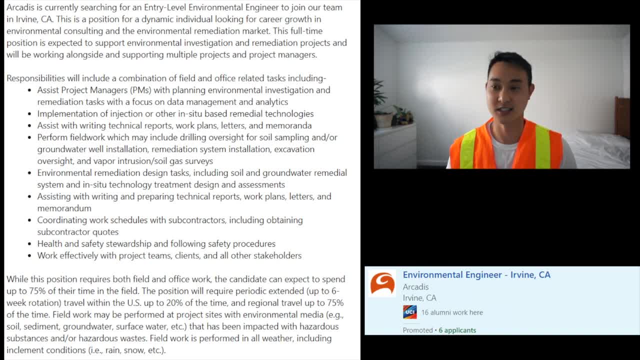 And most of my time working here. at my current position, I'm not out in the field. I don't even have soil sampling experience. So they might say, like you know, you don't have this experience, You might not be well qualified for this job, Even though I know that it's not as difficult as they. 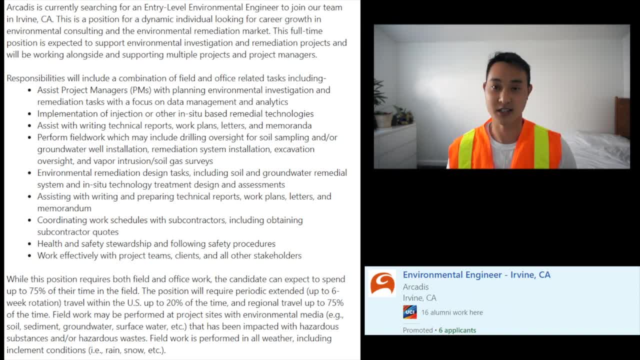 make it out to be. They probably are looking for someone who is pretty active or has had experience before that. You know, they don't want to hire someone who doesn't know what they're doing, So I'm looking for someone who is really good at cleaning up my mess. You know, I don't think they're. 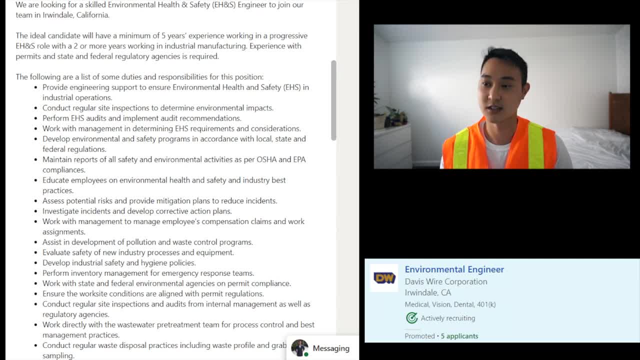 gonna choose an engineer because they're agile or街 안, but I do think you're looking for fine engineers. Now the next one: environmental engineer from Davis Wire Corporation. It's a company located in Irvingdale, California. You are looking for a skilled environmental, health and safety. 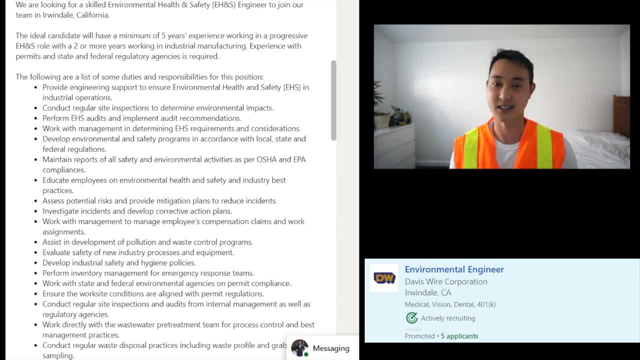 engineer. So right off the bat, EHS an engineer. This is not an environment engineer, It's towards like health and safety. You might be thinking like what's the difference? It's not really. you're gonna be doing like audits, inspections, and like just looking around at the facility saying, oh you know, I see some wires that are like 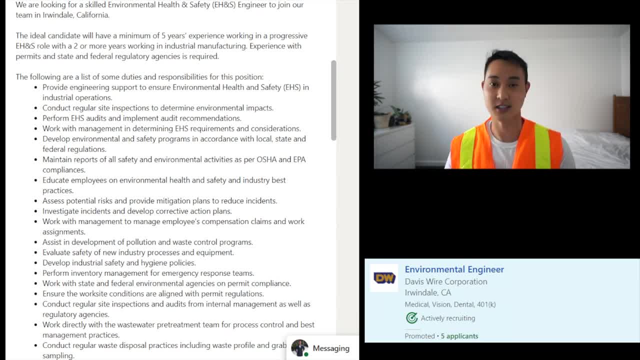 Exposed it might be dangerous people. It's really towards like safety, not so much like Technical skills, if that makes sense and they say the ideal candidate will have like a minimum of five years experience. Let's be real here. No one has that, or you know. 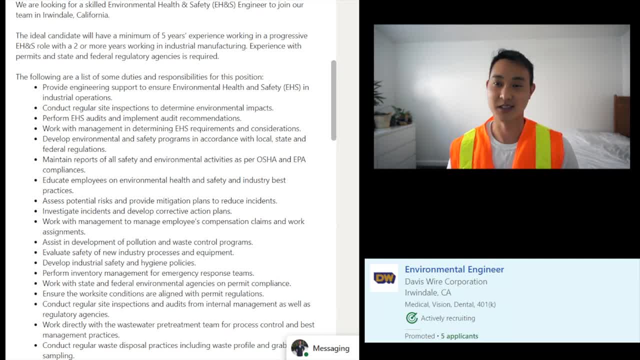 Not many people have that going into this field, like you're not gonna be coming out graduation with like five years experience already. So like this is what I frustrated me about: jobs must be the responsibilities. So first one will provide engineering support to ensure Hs and industrial operations. so again, really towards safety, not really towards the environment. conduct regular site inspections. 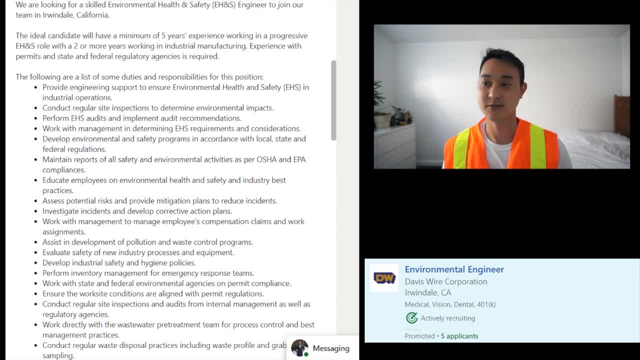 So this is what. I went off and said that you're gonna be going to the field. I'm looking at the site more so than like working in the office or like your computer Trying to design and draw all these lines and circles. Let's just skip some more, because there's a lot to read here. 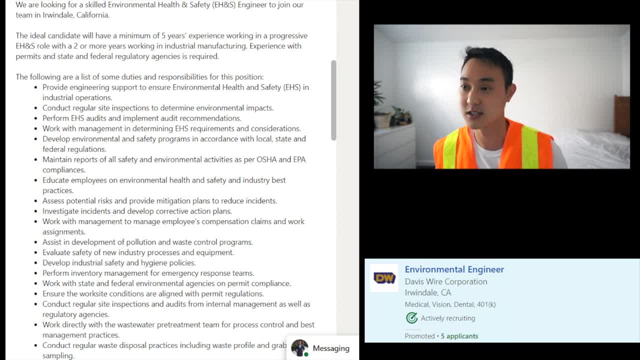 Maintain reports of all safety and risk Environmental activities as per OSHA and EPA Compliances. so let's paperwork Educate employees, assess potential risk. So again what I mentioned about, like those wires being exposed, assist in development of pollution and waste control programs. Evaluate safety of new industrial processes. I'm gonna skip down more and more. 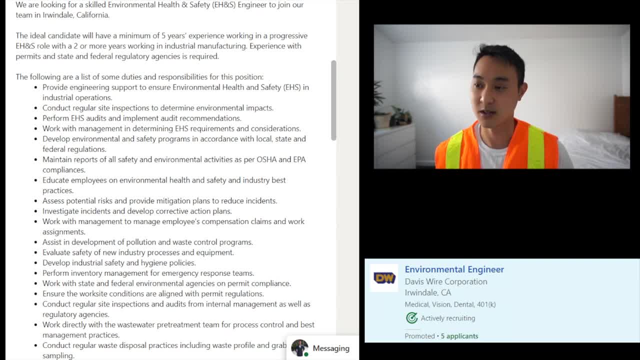 So sorry if I'm going too fast. work with state and federal environmental agencies or permit compliance, So again permit Ensure. the work conditions are aligned with permit regulations. So permit again. You know I'm writing the permit, but you do have to look at the permit a lot and I don't really even understand. 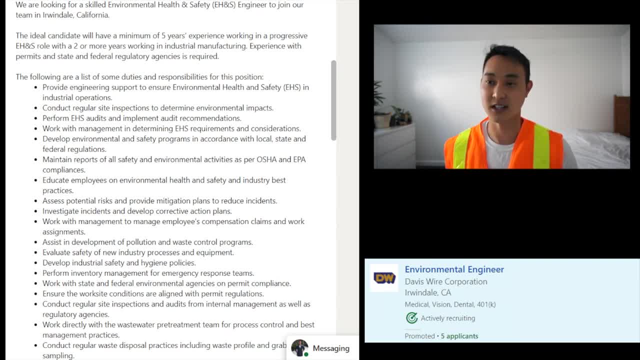 At least for what I have to do like permit writing and regulations. I just know that we have a permit that allows us to do what we can do. It allows us to do what we have to do, but I'm not the one writing it. I'm just giving them from the money and saying: can we do it? Are we about to do this? 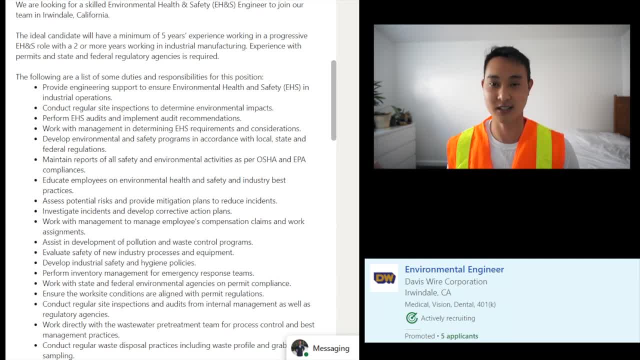 If so, here's the money. cool, Thanks. Here's a piece of paper saying that I'm allowed to do it. I'm not like the one writing a full-on like essay saying here's why We're doing it. Can you please you know like? here's the reason why we're doing it. 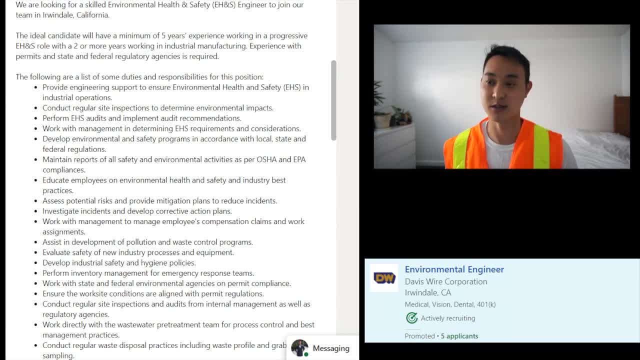 I'm not writing or convincing them to give us a permit. I'm just saying: can we have the permit and then they'll figure out whether or not we can do it or not. But this is just my role. So if you're into the permit writing, You know. 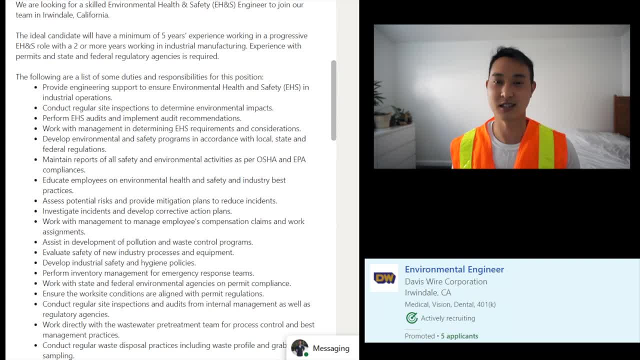 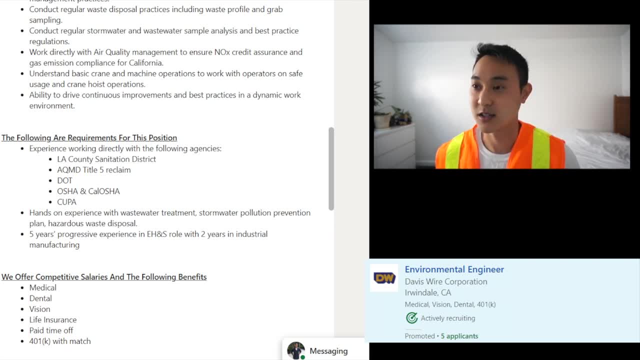 Please leave a comment down below and like, just explain to me the process of it, because I don't really know that much of it. So there's a go really long. this chance, you know, Jump straight down, yada, yada. conduct regular stormwater and wastewater sample analysis. 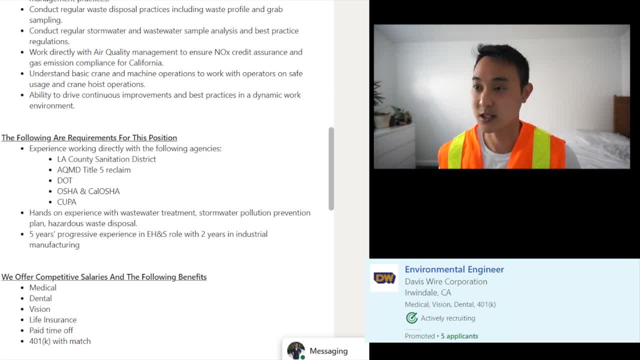 So give me working a lab again For this one too. It's a lot of work. work directly with air quality management to ensure Knox credit assurance. understand basic train and machine operations. That's a bit dangerous. That's, you know, Pretty more intense than currently all the job positions that I've looked at. it require you to do the following. our requirements for this position: 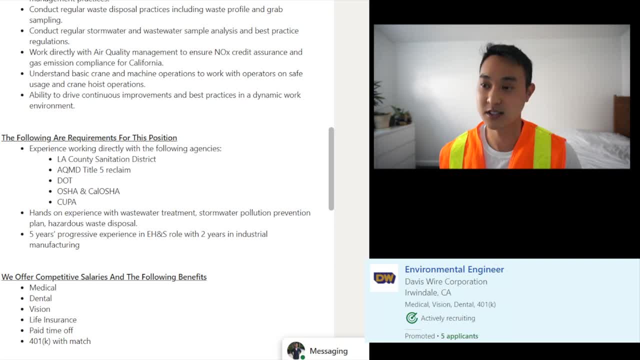 experience working with LA County Sanitation District a QMD, DLT, OSHA and Cal OSHA Cooper. he's not experienced with wastewater treatment, stormwater pollution prevention. five years of progressive Hs role with two years of industrial manufacturing and you know they offer all these benefits for, you know, working there. 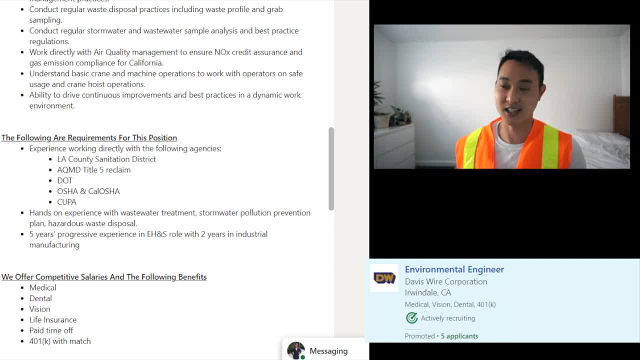 All right. So straight off the bat with this one. I know if I apply I will definitely not get in. so they're expecting like five years of experience and they want all these responsibilities and they requirements. so unless you are Very experienced and you've had all these things, You really have no chance to be honest. 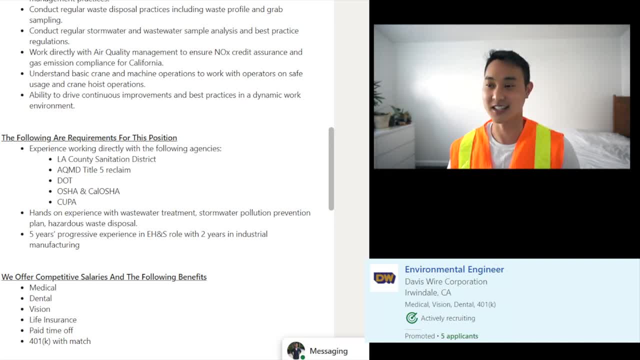 I have no chance at all tears, So don't get like affected if I'm saying that you know you're not good enough for the job. I know I'm not good enough for this job. Of course, with longer years of experience you're more likely to fulfill all those requirements, or you've might have been exposed to some of these. 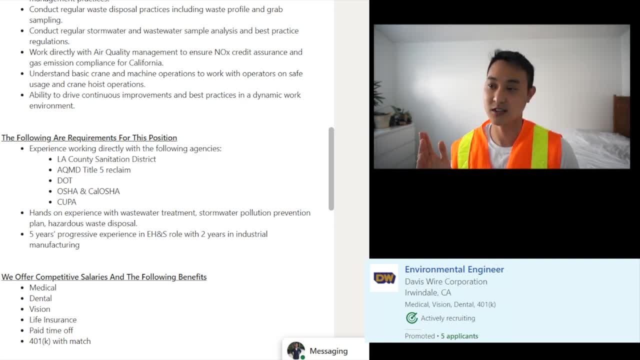 I know I've been exposed to like at least half of them, but I know deep down that I don't know how to do More than half of these two like air quality, stormwater regulations. I don't have that much knowledge in like safety audits either, because I'm a position like I am- an environmental engineer. 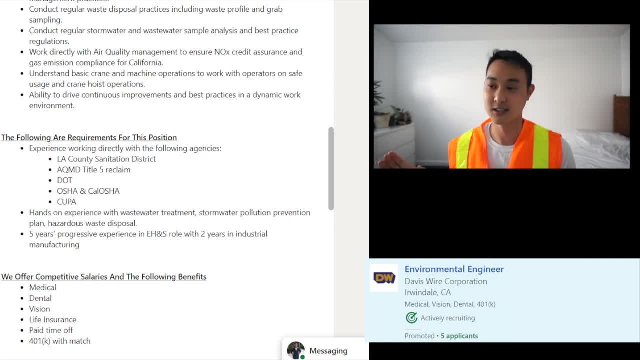 But we also have a safety engineer, So like there's two different roles at my job. Well, this one job is saying let's combine both of them into one. So I do feel sort of bad In that if this one person has to have so many responsibilities, or just you might be overworked. 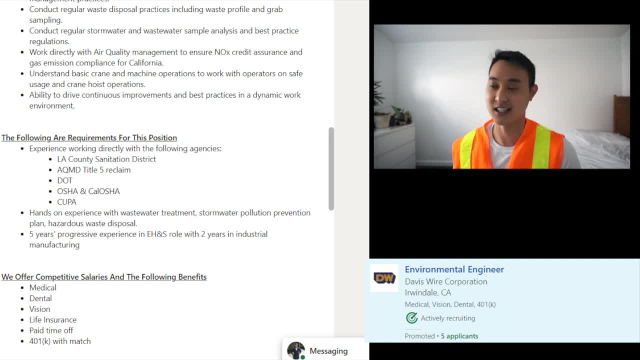 And the end. I hope that this guy's getting paid well for what he does, because that's a lot of responsibilities, a lot of requirements, a lot of things that can go wrong and if he doesn't, I guess, Perform well, it might affect them. moving on, I'm looking at a staff: environmental compliance consultant associate-level. 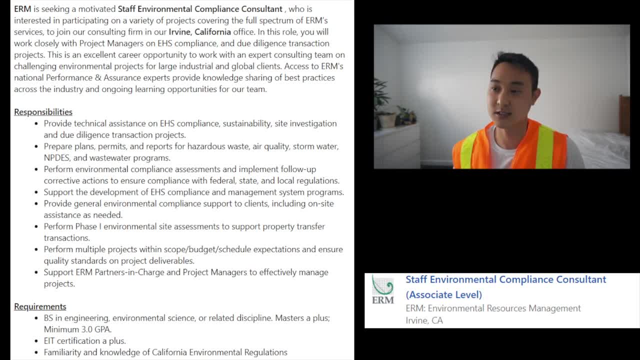 companies from ERM Environmental resources management, so I've heard of them. They're pretty big. It's located Irvine, California. let's see what their responsibilities are. okay, so not so much as the last one. they need to provide technical assistance on EHS compliance, sustainability, site investigation and due diligence transaction projects. so 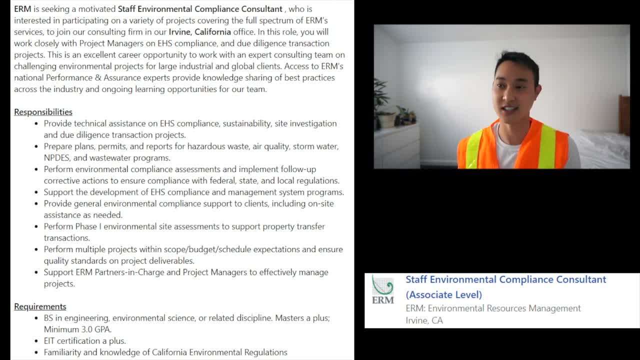 you see how right away they're sort of they separated, at least for this one, this position- environmental compliance consultant- with the EHS person. so, just like my job, we have two different people doing two different things, while the other job that I just mentioned- the whole long list- had one person do two. 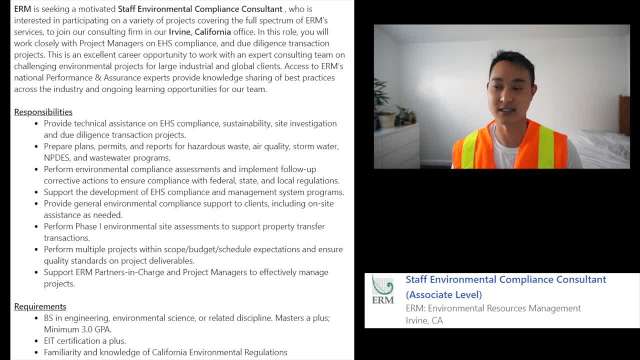 people's job, so again that guy can be overworked. I think it's just much easier to have two separate people doing two different things just working together. the next responsibility is preparing plans, permits and reports for hazardous waste, air quality, stormwater, NPGES and wastewater programs. I do 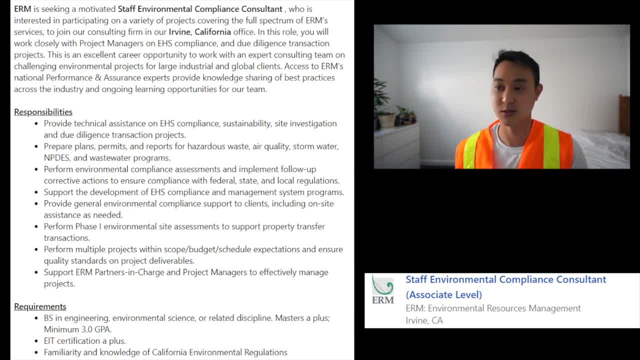 hazardous waste, but for this position they're doing like much more than that, so they're probably handling the entire field, as compared to me, where i only like handle at least a fraction of those fields. they perform environmental compliance assessments, collective actions to ensure compliance with federal, state and regulations. 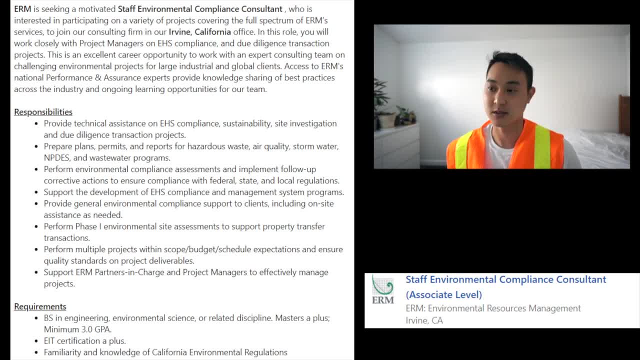 support the development of ehs compliance. provide general environmental compliance support to clients, including on-site assistance as needed. perform phase one environmental site assessments to support property transfer transactions. perform multiple projects within scope, budget schedule expectations and ensure quality standards on project deliverables. requirements are to have: 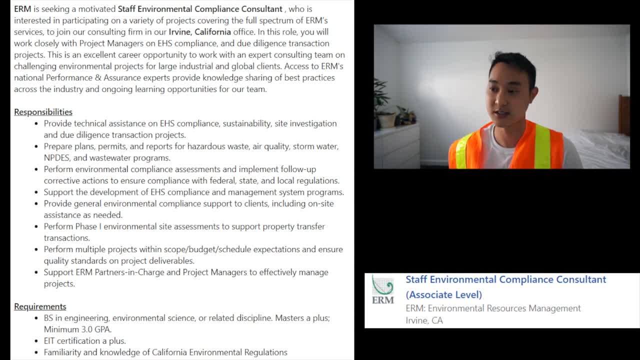 like bachelors in engineering, environmental science or related discipline. you know, masters is a plus, mineral 3.0 gpa. i honestly don't believe they're going to check your gpa. but whatever, eit certification is a plus. familiar with california environmental regulations. okay, i'm sort of confident that if i were to apply to this job with my current experience, okay. 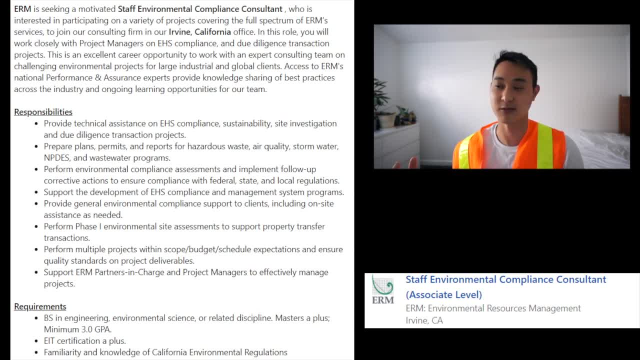 not not just me like graduating right off the bat, but, like with my two years of experience, i probably would be able to transition pretty well into this. i just don't know that much about the air quality, storm, water quality and the other things that i would be able to transition to the 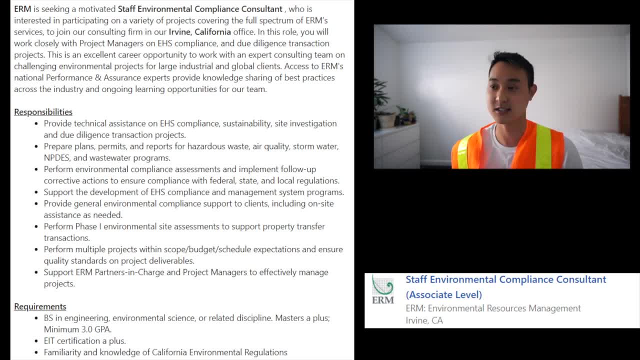 and other wastewater programs like those permitting and those things. but in terms of like what I do right now with like meeting up with compliance regulations and just writing reports, I do have experience with that. all right, so that's good. I'm not so far off. I can still like. 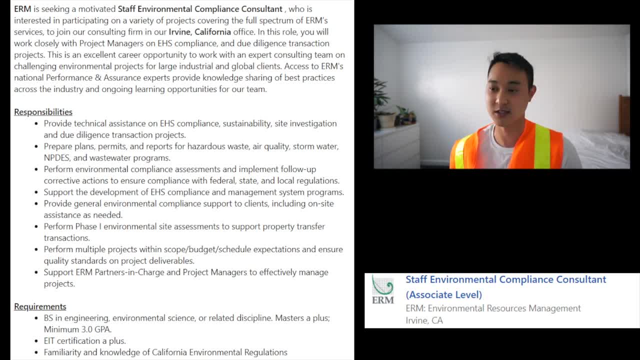 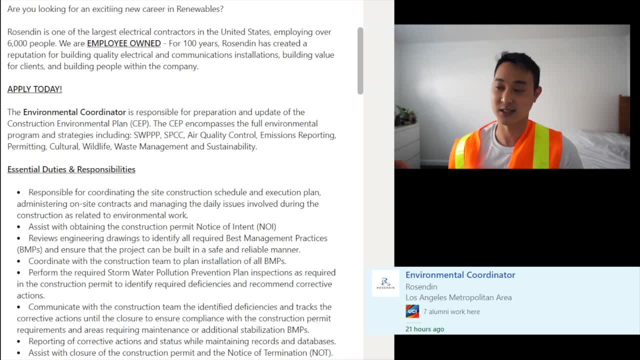 be hireable if I get fired at my work and I do have like some of those requirements already, so it's not so bad in that I can actually meet the expectations. so on paper I look good. and the last one, because I don't want this video to be like so long and just have me ramble so much. the last one. 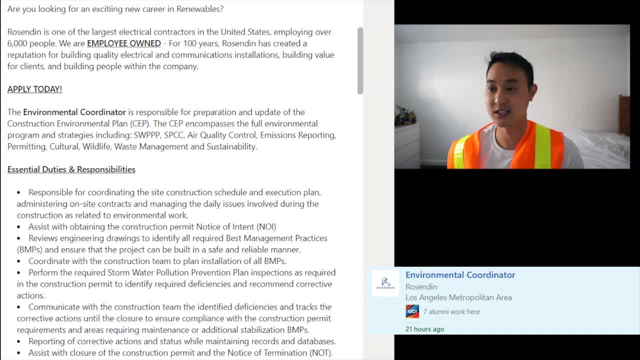 is an environmental coordinator. the company is from Rosenden, located in Los Angeles. if you have that for the most part environmental engineers or like coordinators or compliance officers or whatever you may call it- they only have one environmental engineer for their entire program. so you might be a bit overwhelming because if it's a small company they might only need one. 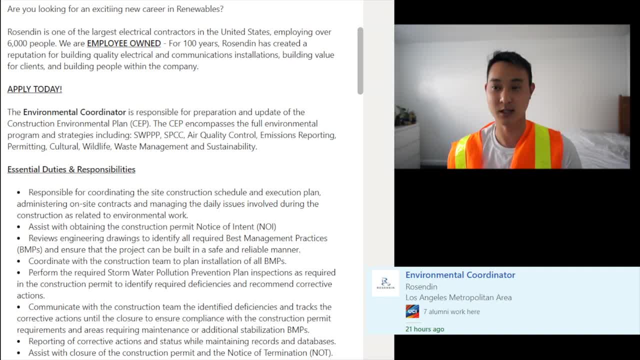 person to do it. so you're expecting like to be collaborating with other people or you might have like five other environmental engineers working alongside you. that could be not the case. you could be working with one person and you might have like five other environmental engineers working alone. just, you know, have co-workers who are in the construction or different fields, but you're 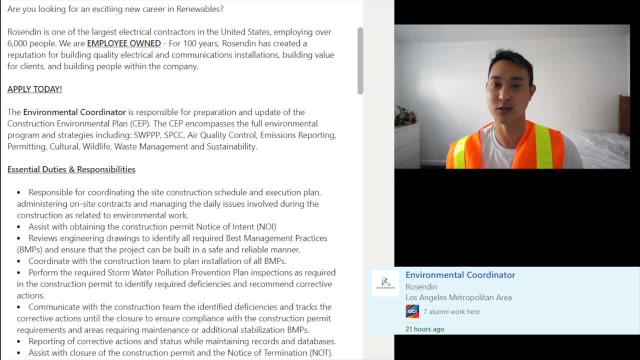 gonna be the only one handling all of the environmental programs, which again might be overwhelming because you're gonna be dealing with so many sectors, so many different programs and if you know one thing goes wrong or you have, like, different things happening all at once, it just might be overwhelming for you. let's look over the essential duties and responsibilities. 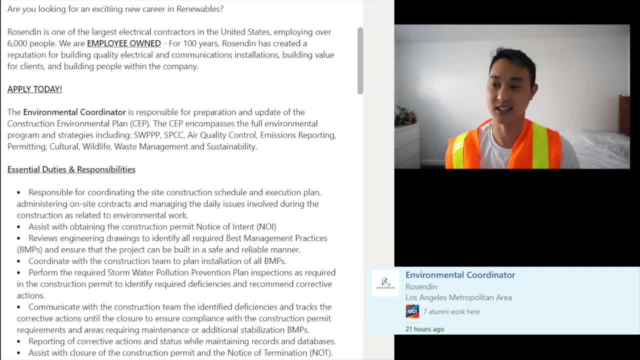 so I'm gonna be skipping around pretty fast because I don't want to talk too much and you know you can read it. basically they're responsible for coordinating the site construction schedule and execution plan. so again, just meeting up with project managers and seeing before construction like what's happening, managing the daily issues involved during the construction as related to 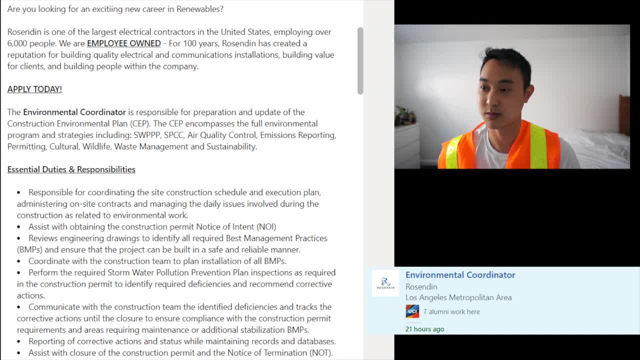 the environmental work. so again, what I just said, assist with obtaining the construction permit, notice of intent, permit writing. I don't have any permanent writing experience up. that already sort of decreases my chance already of like getting into this position if I tried to apply coordinate with the construction team to plan installation of all BMPs. BMP stands. 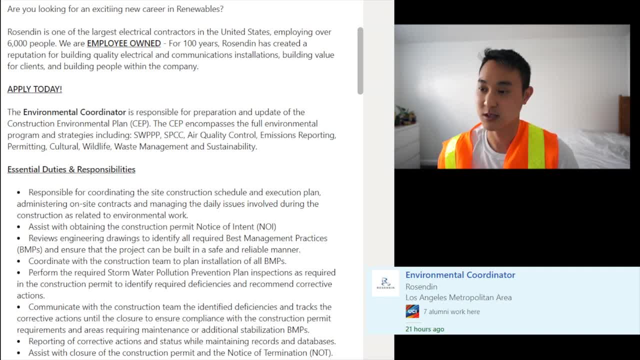 for, like business management practice, perform the required stormwater management practices. stormwater pollution prevention plan inspections are required in a construction permit to identify required deficiencies and recommend corrective actions. so if you're not really aware with what that means, it just means that you have like a plan, basically before people start digging up. 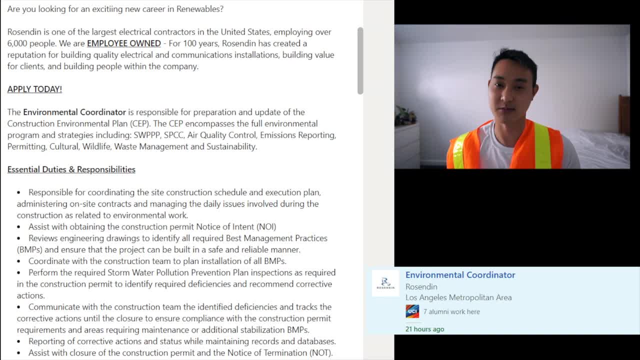 dirt and like breaking up stuff. you have a piece of paper you just do like maybe 100 pages long worth of like here's what can go wrong. and if it does go wrong, here's what to do. just a plan. so you'll probably be reading it saying, okay, uh, there's like the storm drain right here next to. 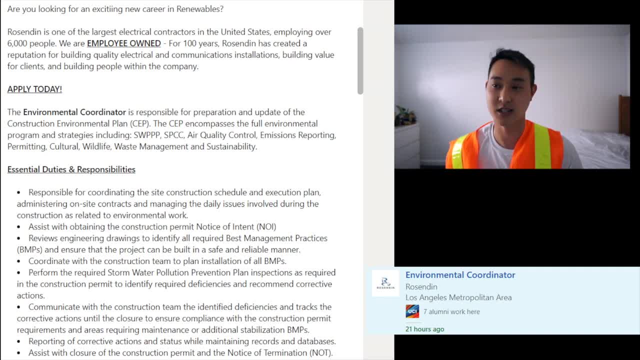 this house, but I want to break the house, I want to demo the house and then, you know, clean it up. but some things can go in that storm drain. so you want to make sure that the drain is, like, properly protected. you don't want junk and like metal and all these toxic substances to go in a storm drain. 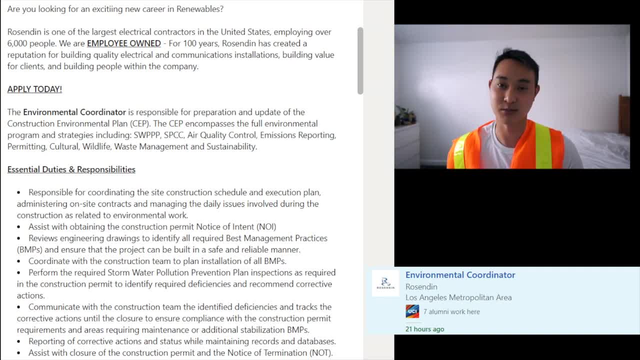 and like: kill all the dolphins, right? so you who are reading the this plan, or you, you who are coming up with this plan, have to find a way of how am I gonna keep this drain protected before, during and after the construction, because sometimes you know everything looks good on paper once you actually 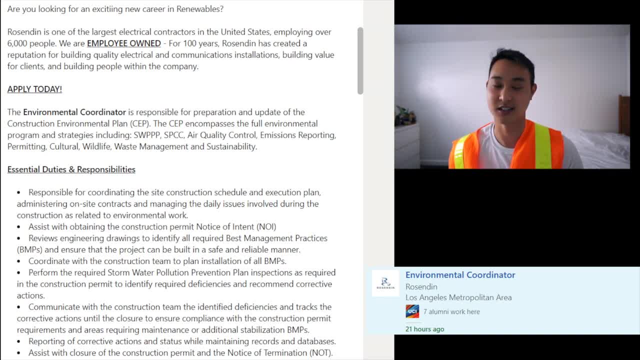 start doing stuff, things can go wrong. and then if something does go wrong, then it'll be falling on you and your responsibilities saying, like you know, I didn't know this, or like I had a plan, but that plan didn't go as expected, as planned, so you're going to be held responsible for keeping 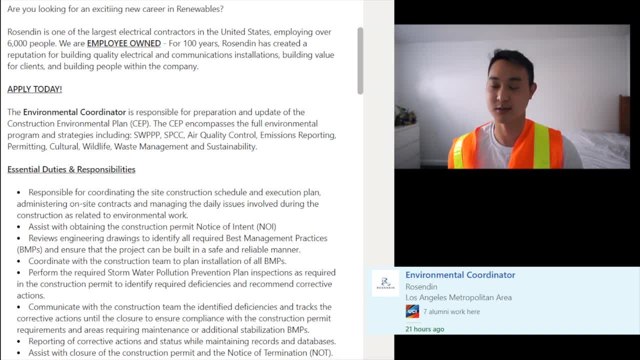 that plan, like all throughout before, during and after the construction project, and so you're just going to be like visiting them every single day saying, hey, make sure that thing is sealed up and your plan. so this is where you got to be a people, person and you know, according to the responsibilities, 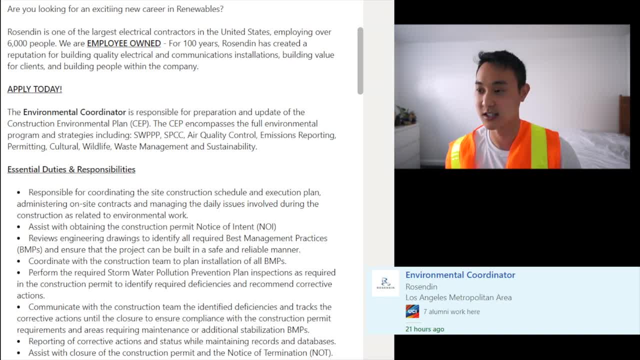 communicate with the construction team the identified deficiencies and track the corrective actions until the closure to ensure compliance with the construction permit requirements and areas requiring maintenance or additional stabilization. BMPs- all that fancy word for you. have a plan, stick with it and don't mess up. basically, that's really all the time today. 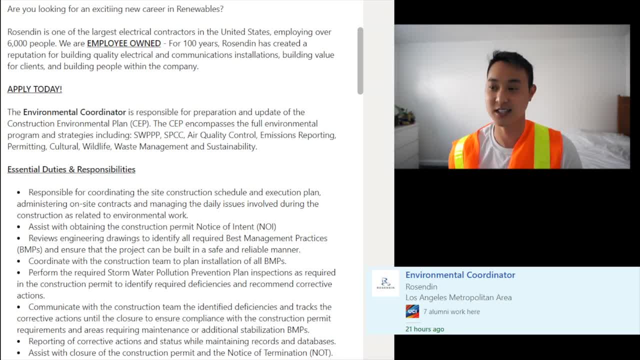 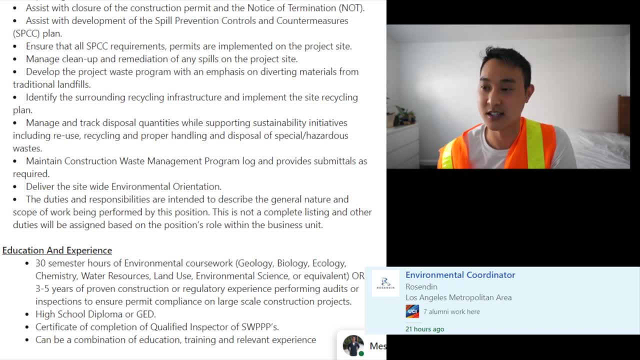 just sounds like more professional. but you know, I'm here to translate in layman's term anyway. so that's what they mean. and the last little point is a pretty funny one, I guess. the duties and responsibilities are intended to describe the general nature and scope of work being performed. 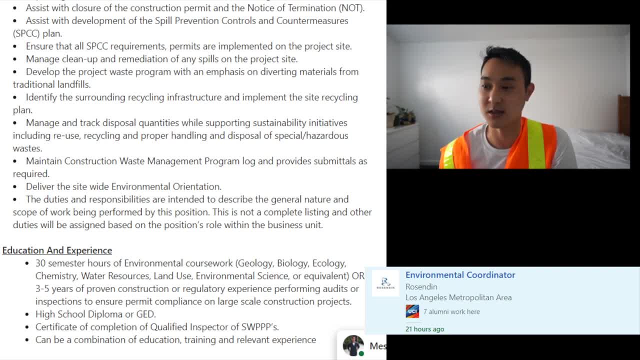 by this position. this is not a complete list and other duties will be assigned based on the business role within the business unit. so that's just the company's way of covering themselves, saying that here's something that you'll be doing, but, like you know, there's probably a lot more that. 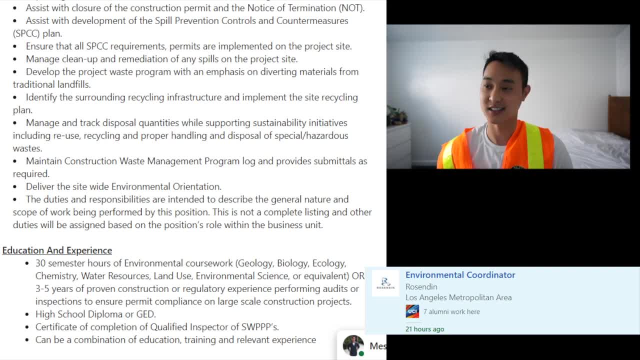 you will be doing. the education experience is not, as I guess, demanding as some other positions. all you need is a high school diploma. sometimes you don't need, like a professional degree, having this sort of physician or role, because you're not going to be so technical on like I need to know AutoCAD to do this. no, you don't. 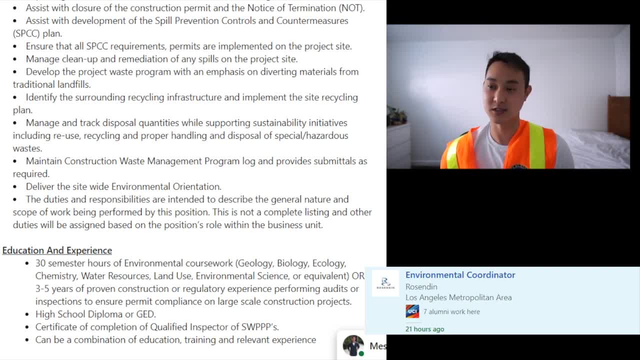 you just need to just be a people person and oversee some site and make sure that, like, no one gets hurt. basically it's more so common sense and ensuring that you know you have a plan anyway. you just got to read the plan and say, okay, let's just stick with it, you don't need to do anything else. 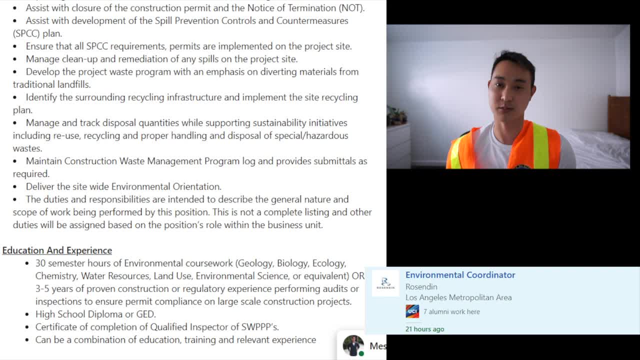 besides, make sure that other people are following the plan. okay, so if I were to apply to this job, will I get it? maybe just because I might feel like I'm sort of overqualified for this, just because I have, like you know, so many degrees and masters or whatever. I have done some of this, but it's not like my specific role. I've done a few of 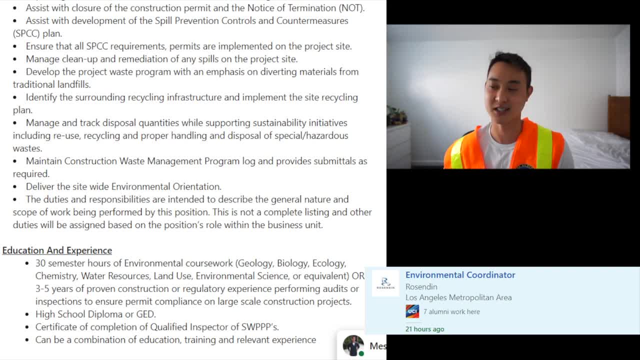 these where I just show up and I make sure that people are following the plan, like making sure that they're not illegally dumping stuff down the drain when I'm not there. or like if I go on a Monday and I see that everything's all sealed up and nice, and then on a Tuesday 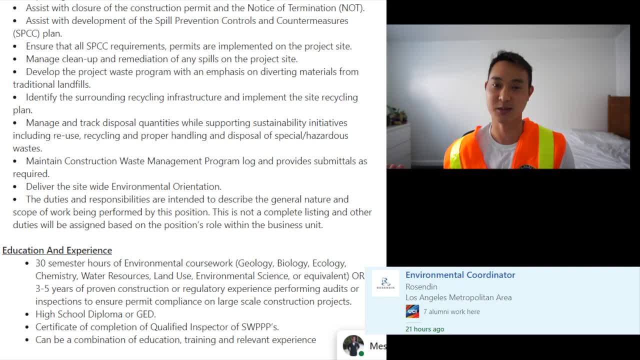 and I see like there's a things leaking down a drain, then I'll be like you know what happened between Monday and Tuesday, like what did you do? why didn't you like suit up? or like why didn't you follow the plan? you sort of have to like be very pushy to those people because I know they. 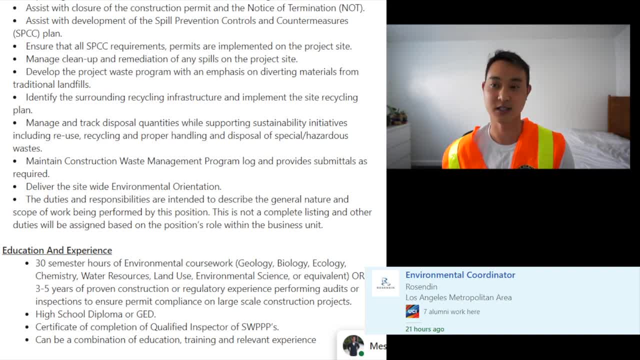 don't really care, they're just here to you know, construct stuff and like finish the project. but you're there to make sure that they finish the project on time but also without like slipping things underneath the rug and you know, follow it in a very professional and like compliant way.